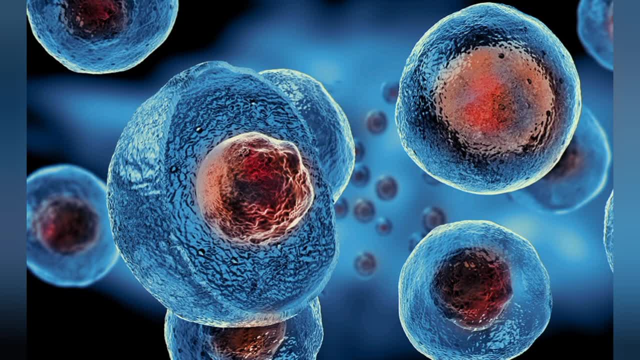 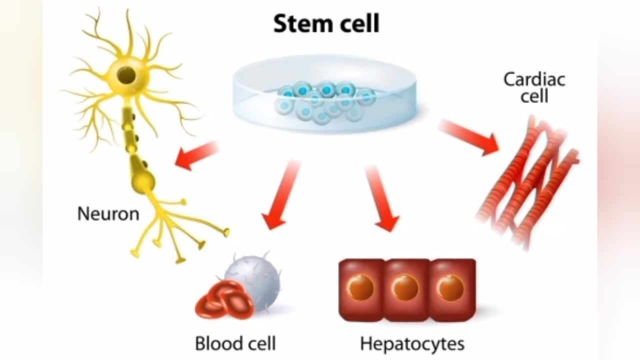 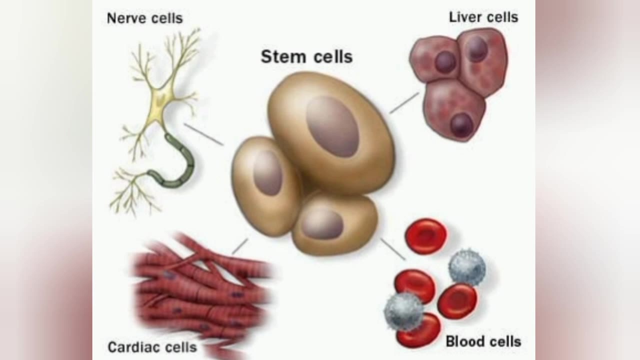 organs and whole body. There are different types of cells for different functions in body. We can say specialized functions, but the stem cell is the cell which can divide into different types of cells and can make different tissues and organs. Stem cell have unique properties and that are- they can divide over and over again to produce new. 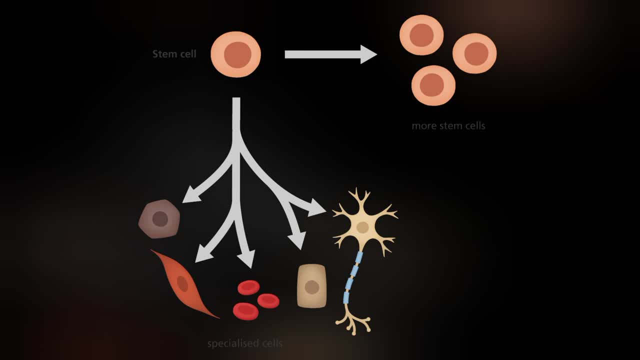 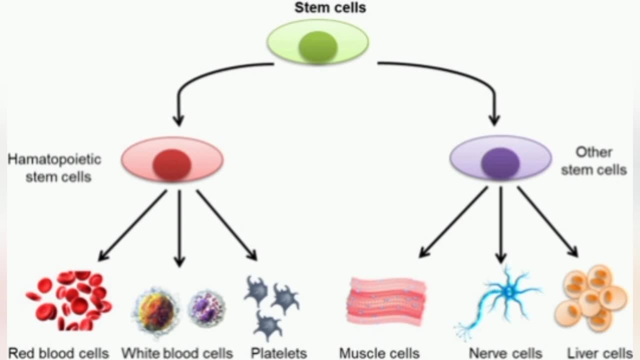 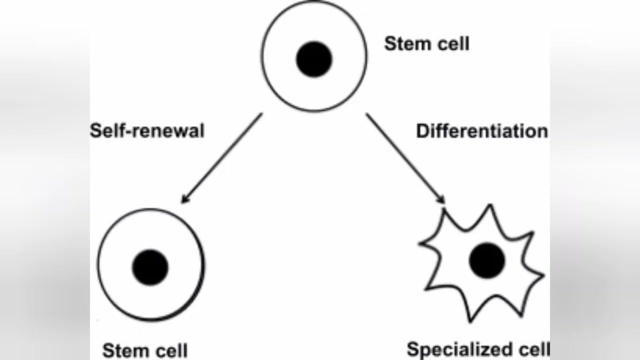 cells. second is they can have potential to develop into many different types of cells in the body, So they can replace and restore damaged tissue. As they divide they can change into other type of cell that make up the body. So by grabbing these properties of stem cells- embryonic stem cells- 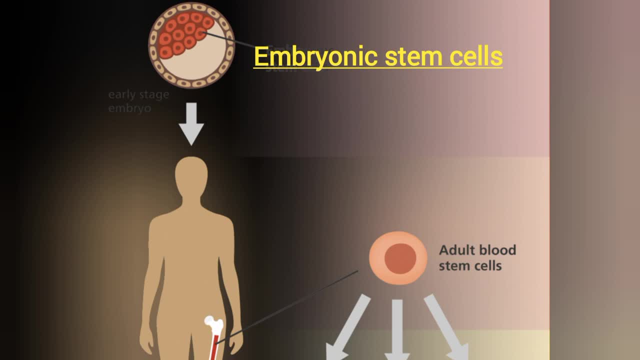 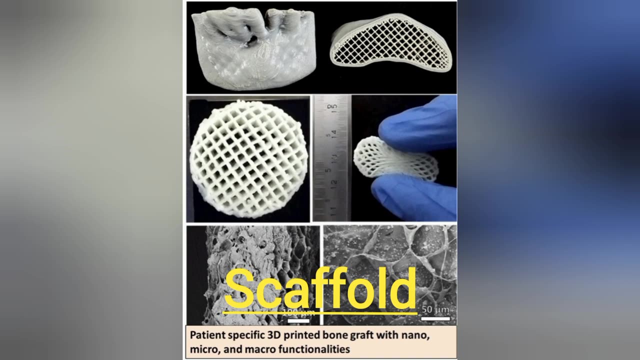 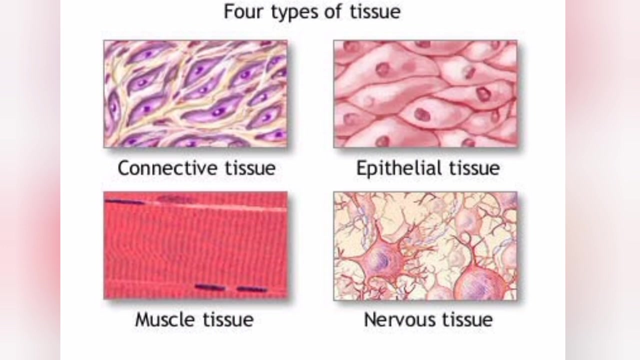 and adult stem cells are used as primary instruments in procedure of tissue engineering. Now next component of tissue engineering is scaffold used in procedure. Scaffolds for tissue engineering are support structures designed to facilitate cellular growth and proliferation upon implantation into the patient. There are different types of tissues in body are connective. 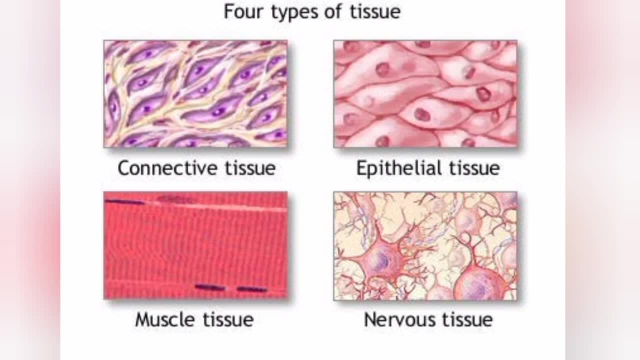 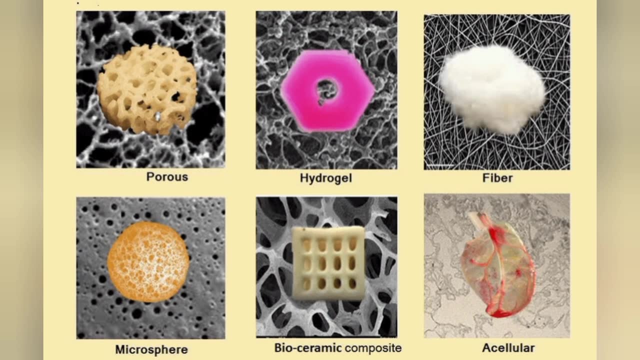 tissue, epithelial tissues, musculoskeletal tissues and nervous tissues. For different types of tissues, different types of scaffolds are used in tissue engineering and are classified in fibrous, porous, hydrogel, microspheres, bioceramic composites and acellular type. The stem cell is also called as: 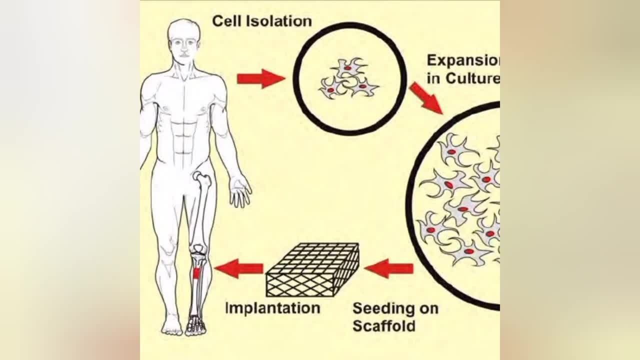 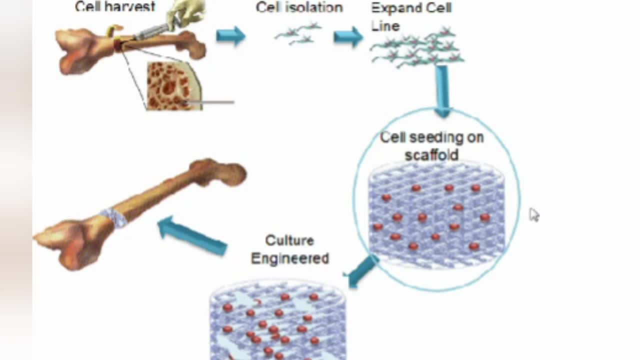 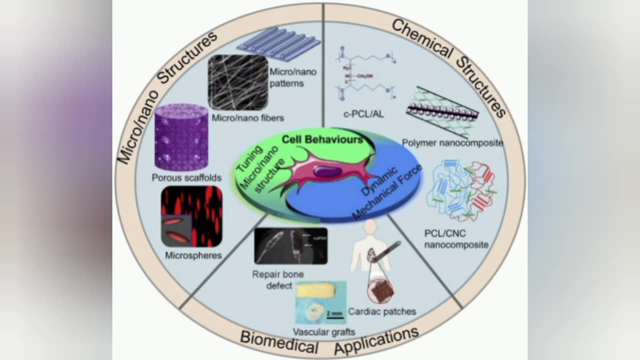 sealed cell and is a starting point of process. Then scaffold holds and supports the seed and steer its growth into desired shape, size and location. Among scaffold materials like polymers, ceramics, metals and composites, each has specific resorption, surface reactivity and biocompatibility properties. Successful implantation requires 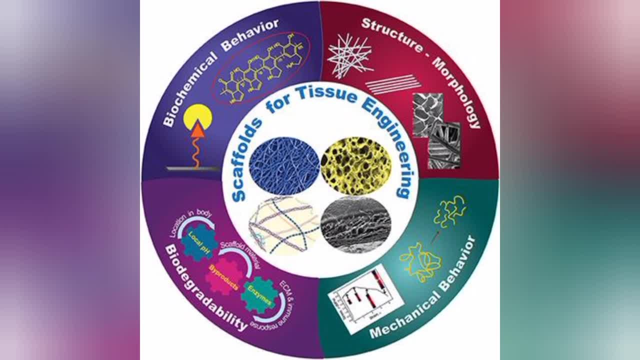 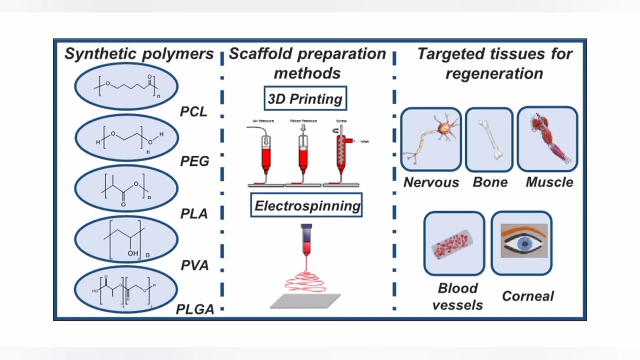 compatibility of scaffold with the host, immunity and functionally integrates with the body. Some biomaterials are extensively applied on large range of medical applications and characterized by good biocompatibility are PLA, polyglycolic acid, that is, PGA, and polydioxanone. This application of biomaterials improves the biocompatibility.